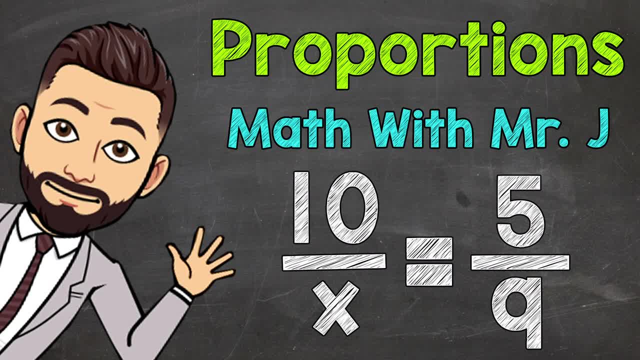 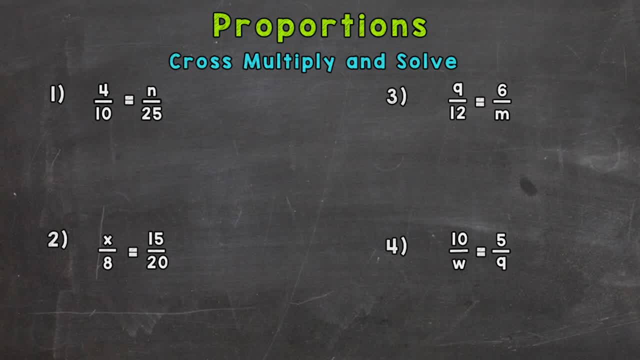 Welcome to Math with Mr J. In this video I'm going to show you how to solve a proportion using cross multiplication. And remember proportions are two ratios that are equivalent and in these proportions we have a missing value represented by a variable. So again we're going. 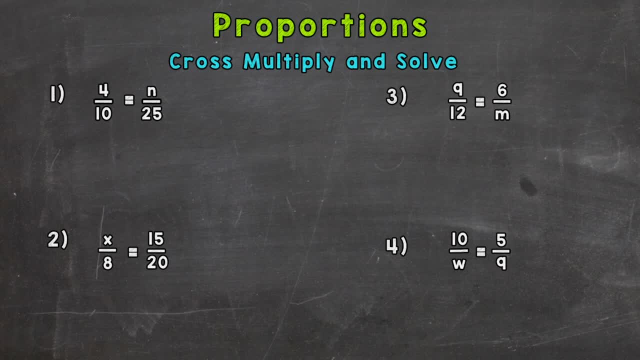 to use cross multiplication in order to solve for that variable's value. So let's jump into number one here, where we have: four tenths equals how many twenty-fifths? So the first thing I'm going to do is draw some arrows to represent my cross multiplication. And now I multiply 25 times. 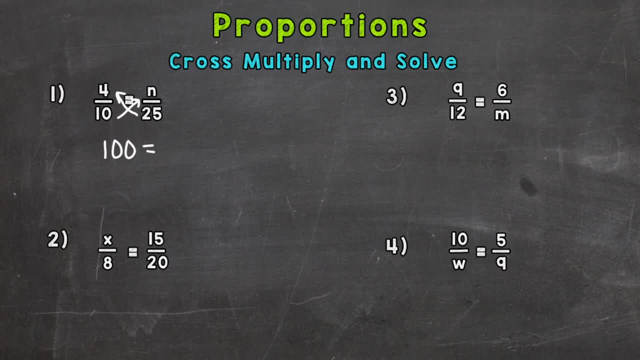 4 is 100 equals 10 times n, which is just 10n. Now it's just a matter of solving this one step equation in order to isolate that n, and we're going to solve for the number one here, where we have four tenths equals how many? 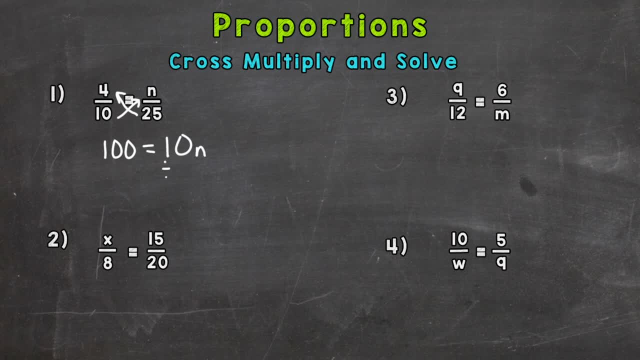 twenty-fifths and find its value. So let's divide both sides by 10 in order to isolate that n and get our answer. So 10 divided by 10 would give us a 1, which is just the same thing as 1 times n. 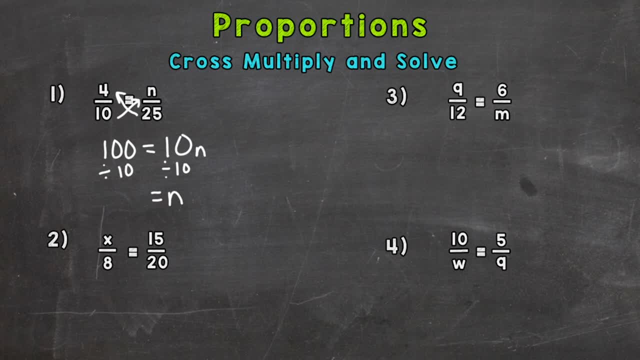 which is n, and a 100 divided by 10 is 10.. So n equals 10.. So four tenths equals 10 twenty-fifths. Number two, how many eighths? equals 15 twentieths. So I'm going to draw my arrows to represent the cross. 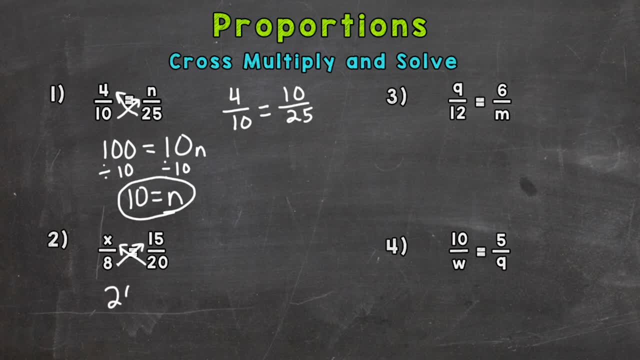 multiplication: 20 times x gives us 20x, and 8 times 15 gives us 120.. So now let's isolate our x and find our answer. Divide both sides by 20 and we get x equals 20.. So now let's isolate our x and find our answer. Divide both sides by 20 and we get x equals 20.. 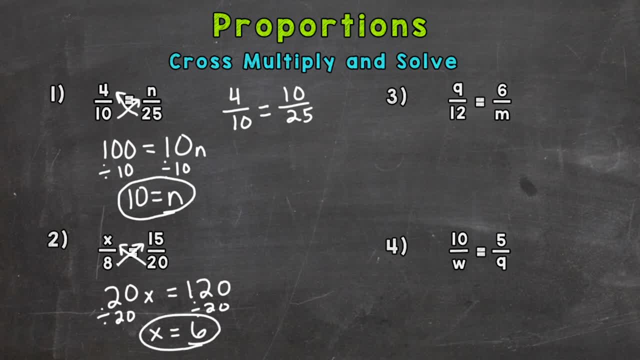 So now let's isolate our x and find our answer, Divide both sides by 20 and we get So on to number three now, where we have nine twelths equals six, and then our variable m there. So we need to find m. Let's draw our lines to represent the cross multiplication.